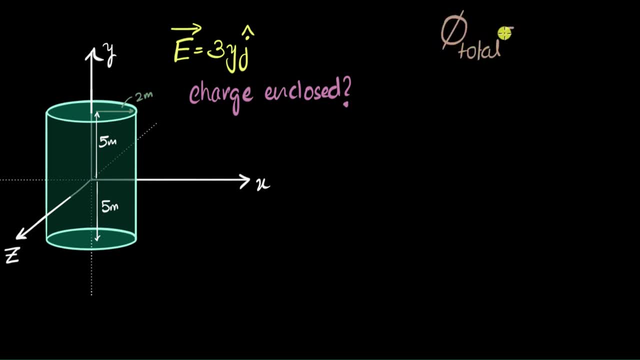 flux through the closed surface will always equal the charge enclosed by the closed surface divided by epsilon naught. And now I ask myself: okay, if I could calculate the total flux through this cylinder, then can I calculate my charge enclosed. Yes, If I calculate this, then the charge enclosed 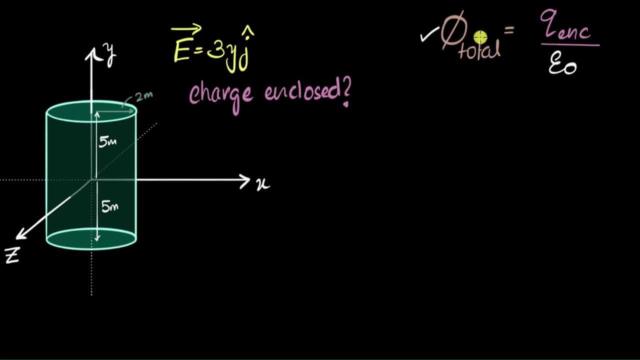 is just the total flux multiplied by epsilon naught, And so I know where to start. now I know my real flux. The real problem is to calculate the total flux through the cylinder. So let's try doing that. So I ask myself next: hey, how do I calculate the flux? Well, if you've seen how to calculate the, 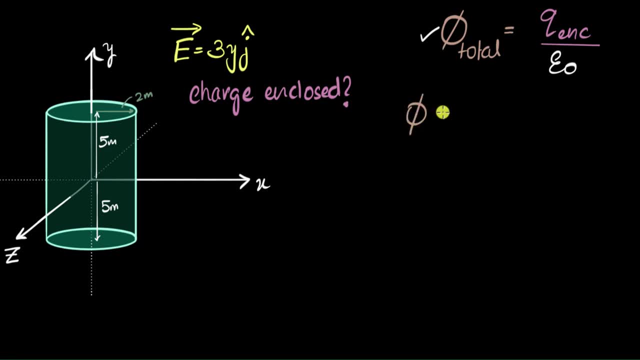 flux, flux through any surface. electric flux through any surface will equal the dot product of the electric field and the area vector. You've seen this in previous videos, right? And if you were to calculate the total flux, then we'll have to do a summation. Now, in general, when we're dealing with, you know, random objects, 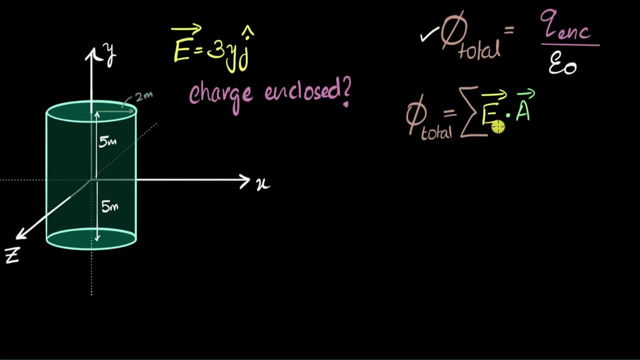 this could be an integral and that could be really hard to solve. But over here I see a cylinder with nice shapes. so that gives me hope that maybe I don't have to integrate. And the reason I get hope is because I can identify three distinct surfaces. I can identify this bottom flat surface. 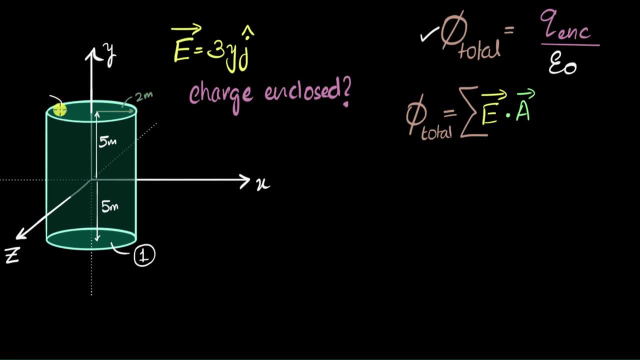 nice and flat surface. let's call that a surface one. I have this top nice and flat surface surface number two. and then I have this curved surface Surface that goes like this, which is not really flat, But let's see what happens. 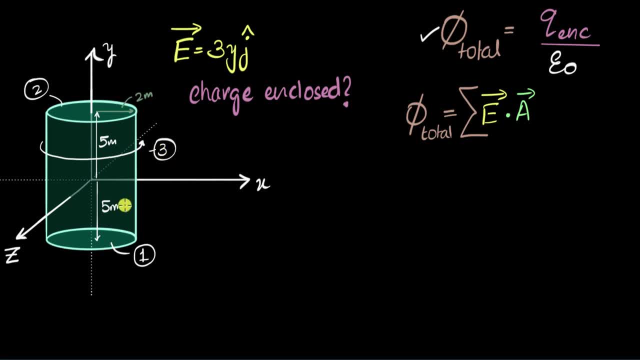 So these are three surfaces that I can identify. So what I can try to do now is try and calculate the flux through each of them separately and then add them up and see if I can calculate my total flux, And then from there I can see if I can calculate. 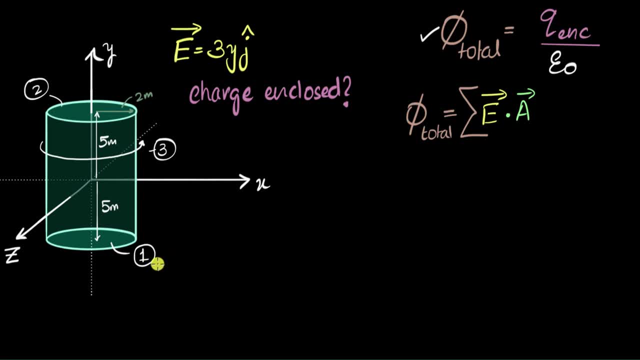 my charge enclosed. okay, All right. so let's see. Let's begin by calculating the flux at surface one. So the flux at surface one that's going to be, from our definition, it's the electric field at that point. 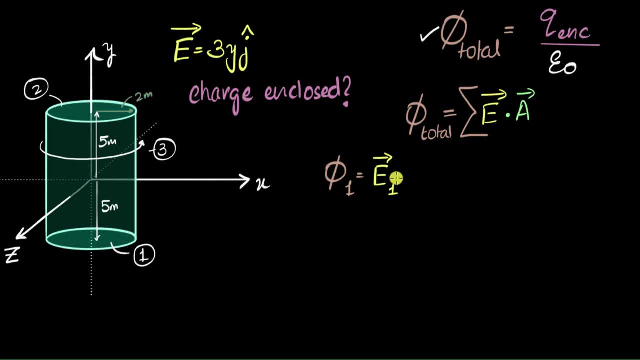 let's just call that as E1, dot, A1, area. at that point- And again, this could also be an integral- if the electric field is changing. so we don't know. Let's see what happens. So I come to this surface and I first ask: 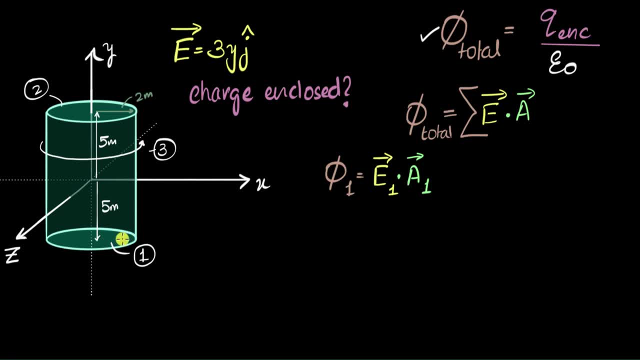 I know how to calculate the area. I know the area is pi r square, so that's not a big deal for me. The question is about electric field. How much is the electric field here? And for that I go back to this scary-looking equation. 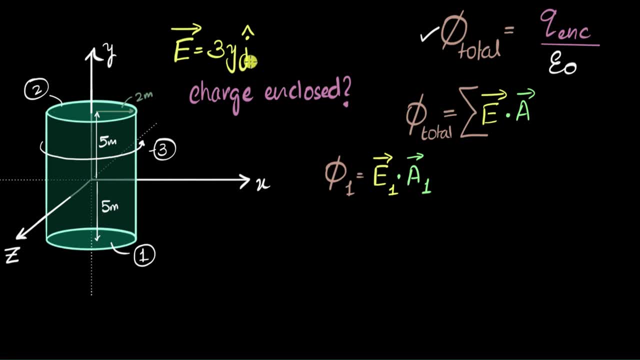 but let's see. So electric field is given to be three: y, j cap. What does that mean? Well, first of all, the j cap is telling me the direction. It's saying that the electric field is in the y direction everywhere. 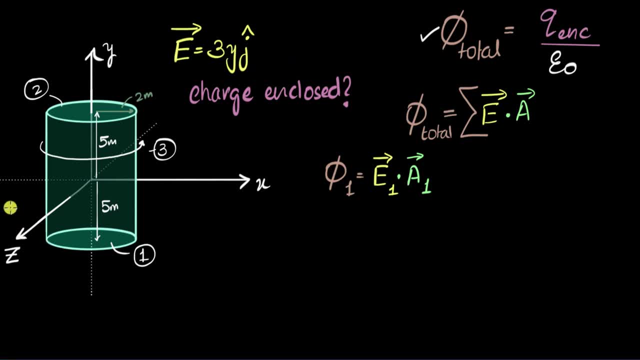 You see, I only have a j cap, I don't have a k cap, I only have an i cap. So electric field everywhere is in the y direction. That's one observation I do, And I can see that the electric field depends on the y coordinate. 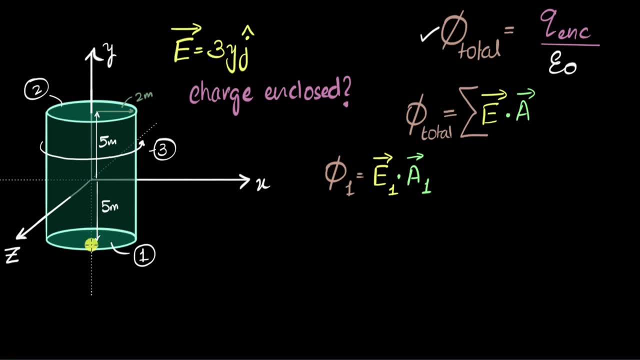 So if I know the y coordinate, I can plug in, I can get the electric field. So at this point, at this point, can you tell what the electric field is going to be? So I want you to pause the video and see if you can figure out. 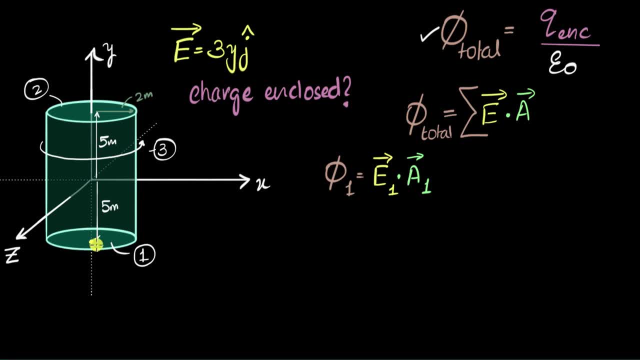 what the electric field at this point is. That's the first step. right for us, All right. So I ask myself, what's the coordinate? y coordinate at this point, That's all that matters to me. y coordinate, And that is negative five. 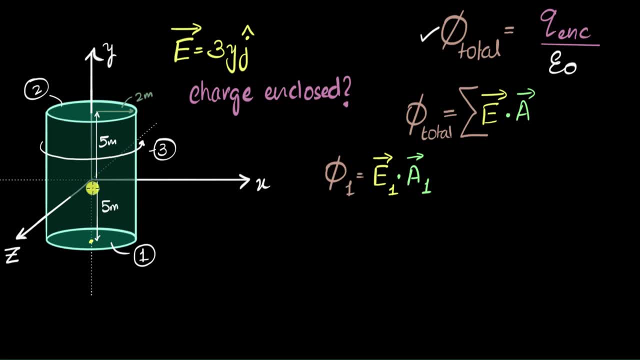 because it's five meters below origin. So upwards is positive, downwards is negative And therefore, if I substitute minus five, I get minus 15 j cap And therefore the electric field at that point, electric field at that point, let me call that electric field at E1,. 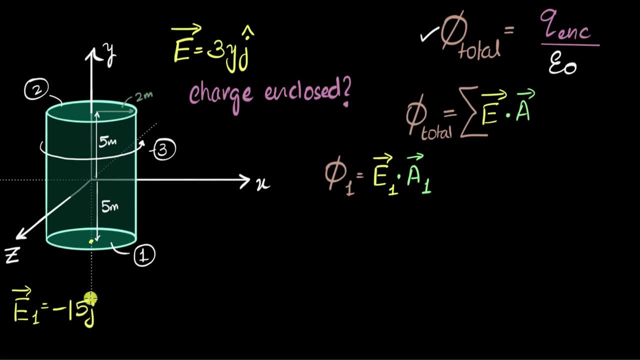 that's going to be minus 15 j cap. And what does that mean? Let's try and visualize. I mean we can just do it mathematically, but let's try and visualize What does it mean to have a minus 15 j cap electric field. 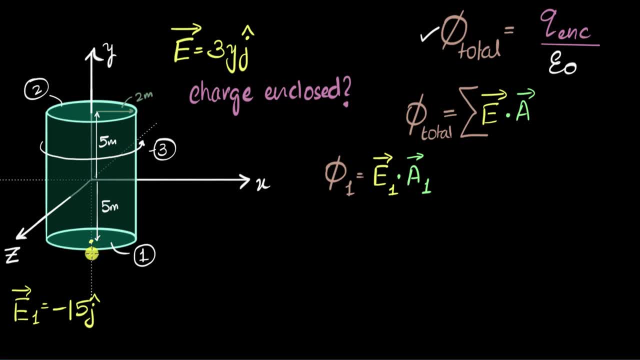 Minus j cap means in the negative y direction, And so that means the electric field at this point is 15 units. whatever the units are, units are not mentioned, so we'll just assume it to be standard units- 15 units downwards. 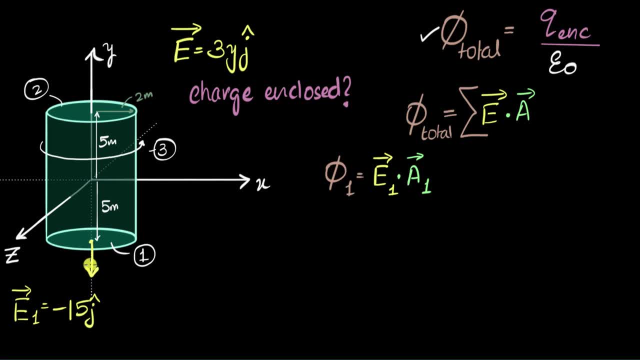 Negative j cap represents downwards. Okay, But I want to know the electric field everywhere, not just at this point, because I want to calculate the flux through the entire area. So what would the electric field at this point? Again, I want you to think about this. 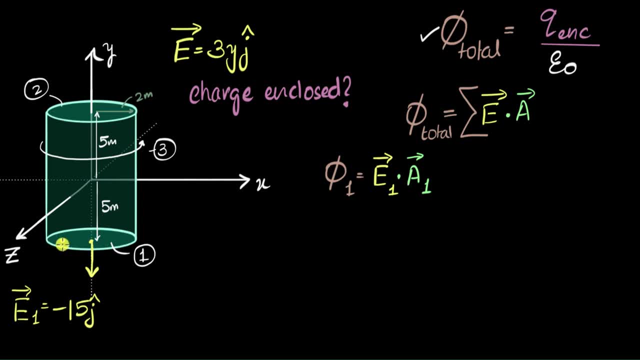 From this equation. do you think the electric field at this point on that bottom surface would be the same, or do you think it would be different? Well, if I go back to the equation, all that matters is the y coordinate. What is the y coordinate over here? 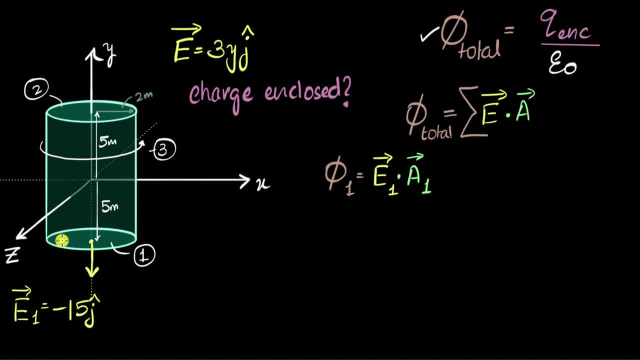 That's again minus five, because again this point is five meters below. The x and z coordinate might have changed, but that doesn't matter, which means the electric field over here is also going to be the same. 15 downwards negative 15 j cap. 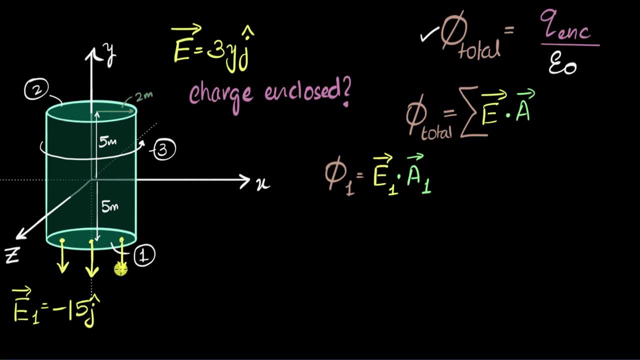 And it will be the same here. So good news, Good news for me, and that's why I'm smiling- is that this is a uniform electric field. Although overall, the electric field is not uniform, It's changing with the y coordinate. 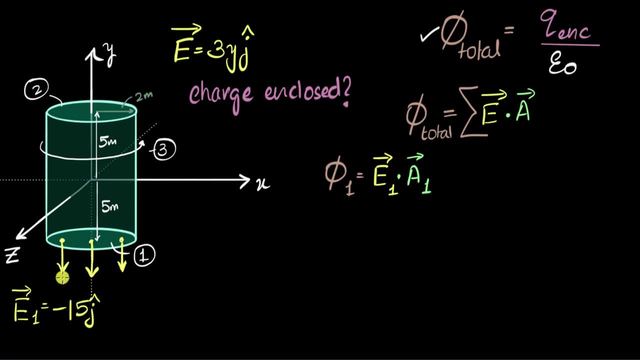 But over this surface the electric field is uniform. It's the same everywhere. That's great because I don't have to do an integral now. Okay, so I know the electric field. Next I have to figure out the area. What's the area? 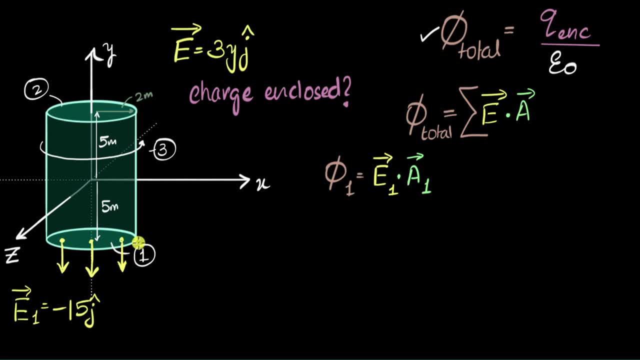 The area is just pi r square. It's given as r is two, So area is going to be- let me just write that over here: area is going to be pi times two. square is four, so it's going to be four pi meters square. 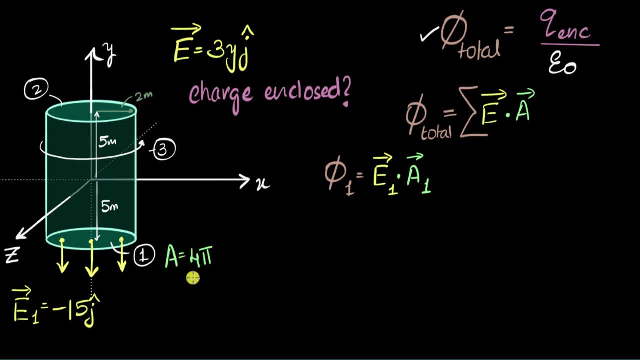 Again, I'm going to write the units, So I'm going to use standard units and I'm just going to keep it as it is. So that's area, But I need the vector area. So what's the direction of this area? 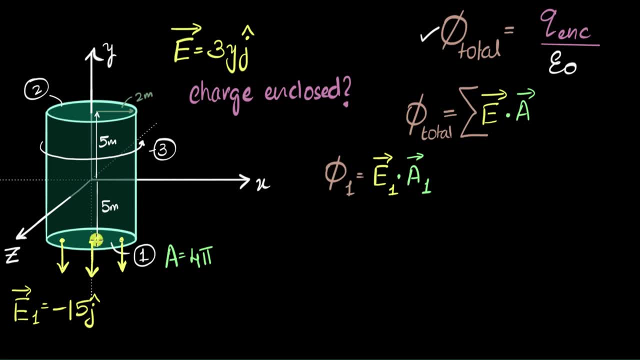 We've seen before how to do that. You draw a perpendicular to it. Now, for closed surfaces, the perpendicular is always pointing towards the outside, So our vector area is going to be pointing outwards. In this case, it'll be downwards. 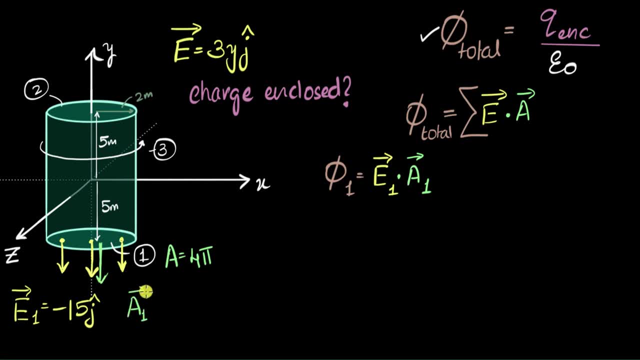 And so if I were to write the area vectorially, it's going to be four pi. that's the magnitude. What's the direction? Direction is negative j, So I will write it as negative j, Now that I have these two. 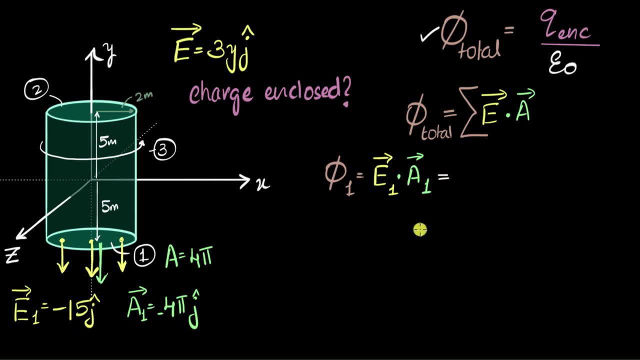 I can go ahead, plug in and calculate what the flux is. And again, good idea to pause at this point and see if you can calculate this flux and then probably you can try and calculate the flux second and third surfaces as well. 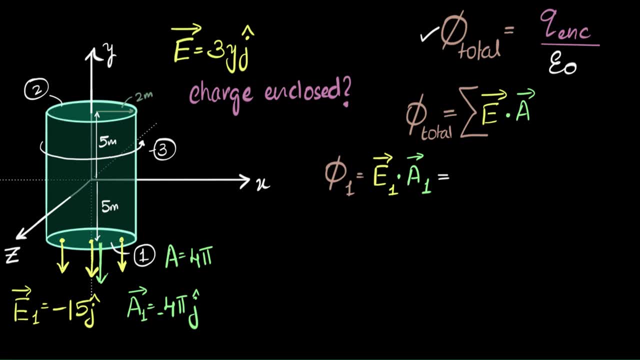 All right. So negative 15 times negative four pi, that's just going to be 15. fours are 60, so that's going to be positive 60 pi And j dot j. this is the vector. What is j dot j? 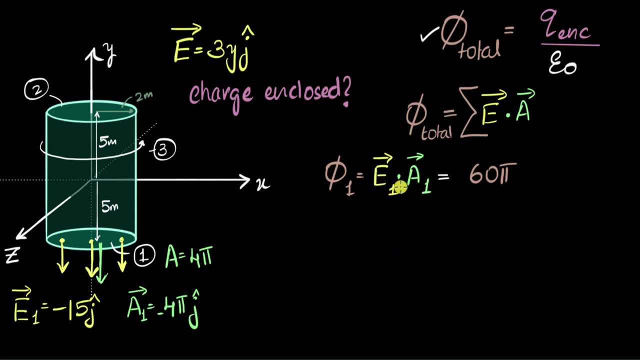 J, dot, j is one. Why is it one? Because dot product has cos theta in it, and j and j means same direction. Theta is zero, cos zero is one, And so you get just 60 pi. That's the flux on the first surface. 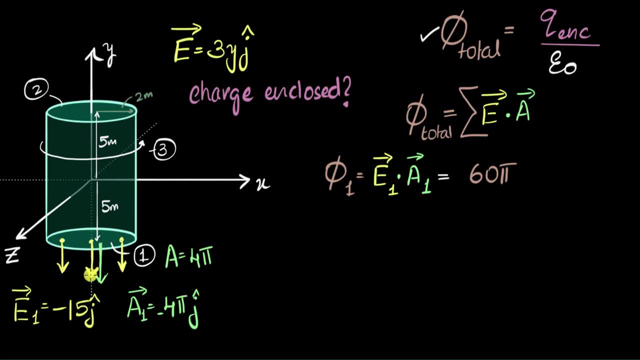 We could have done it directly, without looking at j anymore, because we would just say, hey, they're both in the same direction. Dot product becomes one, and so it's just e times a Could have done that as well, All right. 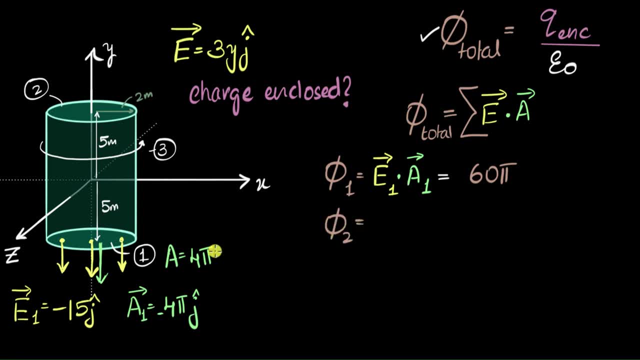 So that's flux through the first surface. We can now similarly calculate the flux through the second surface. Again, what do you think it's going to be? Well, let's calculate the electric field, The electric field. at this point, the y coordinate is all that matters. 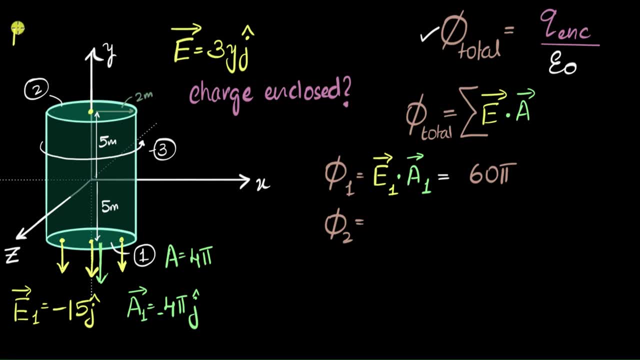 It's plus five, So I get plus. let me see, it's going to be e two, it's going to be 15, plus 15,, j cap. And what about the area? Well, again, the magnitude will be the same: four pi. 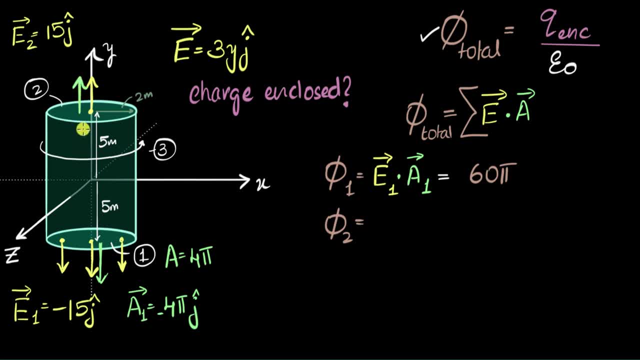 And this time it'll point upwards because, remember, area vector is always outwards. So area a two would be four pi, this time positive j cap, And so if you dot them again, notice you get 15 times four pi, that is 60.. 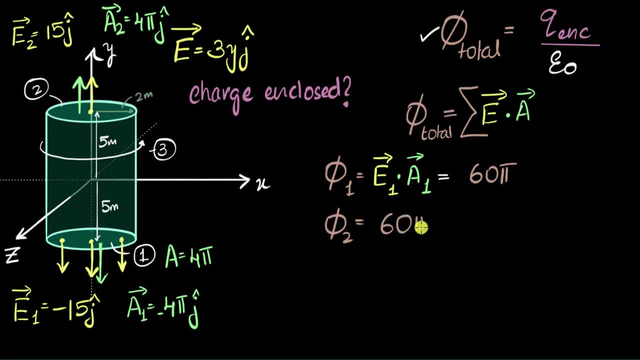 J dot, j is one. So you get again 60 pi. And at this point you might think- and at least I used to think- but wait a second. in one case you're getting upwards, in the second case you're getting downwards. 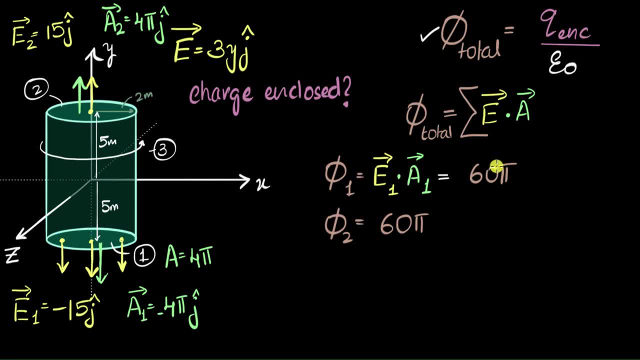 Why am I getting both as positive? Why Shouldn't one be negative of the other? Why is that? Because, remember, flux is a measure of flow. Outward flow is positive, inward flow is negative. So, even though here electric field is going up, 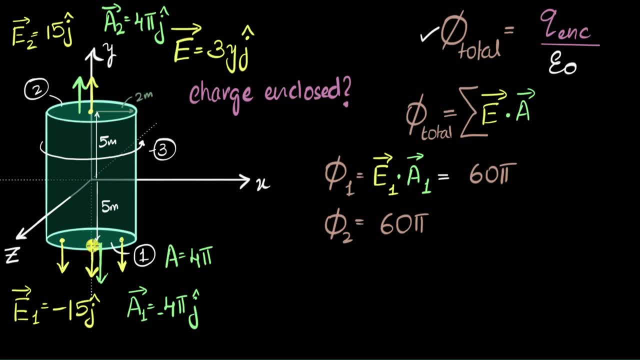 it's flowing outwards positive, Even though the electric field over here is going down, it is going outwards. That's why it's also positive. You get that, So don't get confused, Take some time to getting used to, but outward flow is positive. 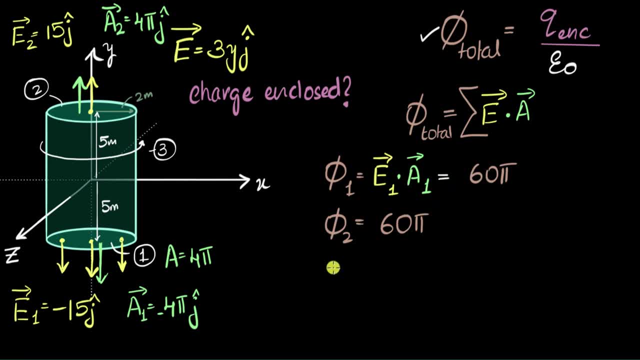 That's what matters. In both cases it was outwards. Okay, now let's go to the third one, The curved surface. And this is the part which looks really tricky, because over here the y coordinate keeps changing And therefore the field is not uniform. 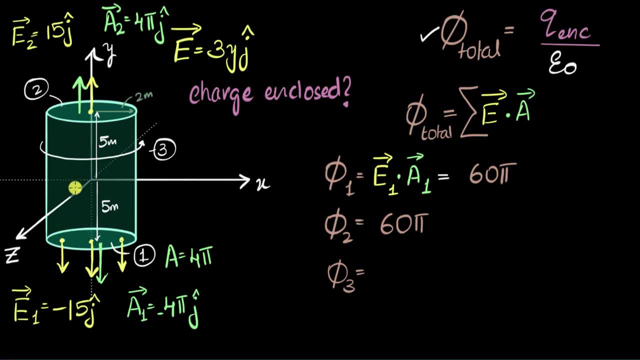 over the entire surface, Oh no. So does that mean we have to integrate? Not really. You see, Again, I want you to give it a try. See what's going to happen. Just look at the electric field's direction carefully. 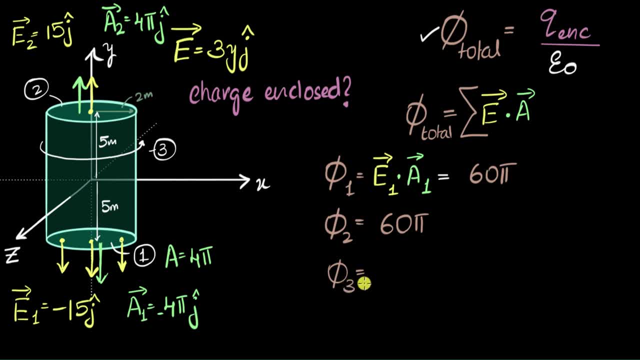 Look at the area vectors that you would draw here And you will see. you don't have to integrate to get the answer over here. Okay, let's do this. So because electric field is in the y direction everywhere here, it's going to be upwards. 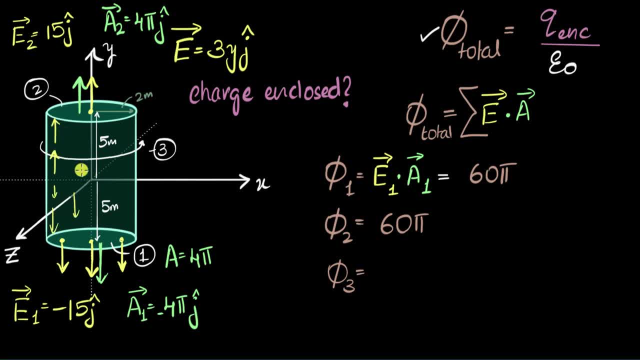 Here also, it's going to be upwards, downwards, downwards, Everywhere. it's going to be upwards and downwards. Below this, it's going to be negative and downwards. Above this, it's going to be positive and upwards. But if you were to look at the area vector at any one point, 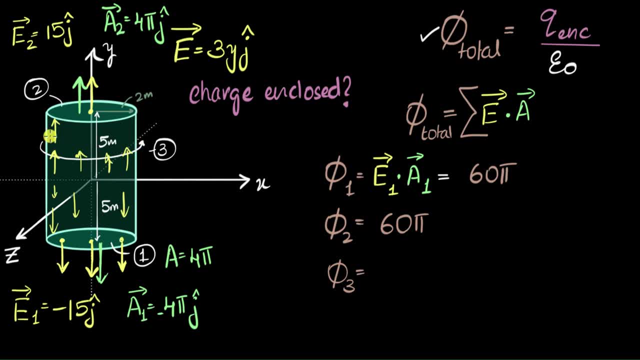 Now you can't draw a single area vector for a curved surface. Whenever you have a curved surface- irregular shape, not flat surface- you have to take small, small sections. If I take a small section and draw an area vector, the area vector will point out this way: 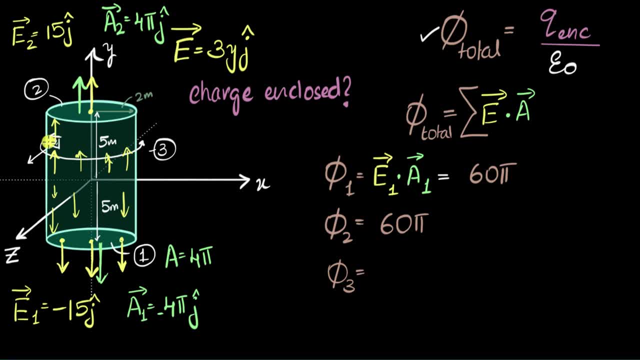 And the angle between the two would be 90 degrees. And that would be the same everywhere. If I were to draw an area vector, it'll come out over here And the angle between this and this would be 90 degrees. And why is that exciting me? 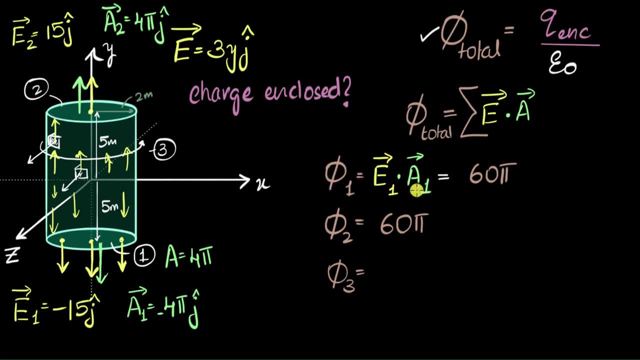 Because that means cos90 is zero. So when you dot it you get zero. So if you were to EA everywhere, you just get zero everywhere And you can logically think about this. Remember, flux is a measure of how much something is flowing out or into that surface. 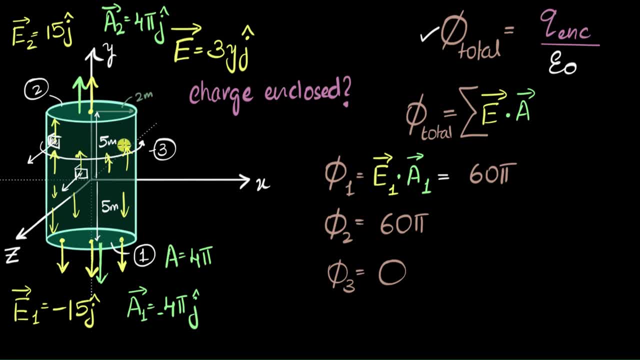 And because the electric field over here is parallel to the curved surface, nothing is flowing out of it, Nothing is flowing into it, And therefore it kind of makes sense that the flux is zero. All right, so now that we have the total, 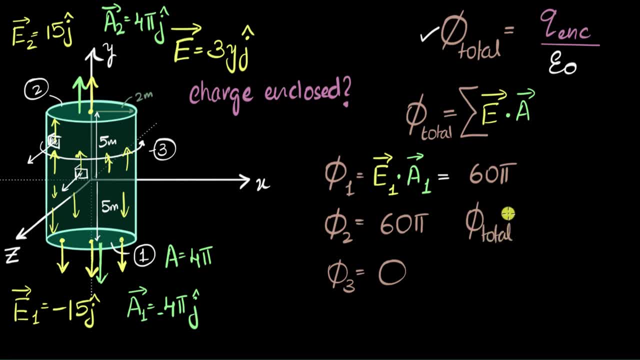 all the flux values. the total flux would just be the summation of all three. That's 60 plus 60,, that's 120 pi, And I can now equate it to charge enclosed divided by epsilon naught. and there I go. 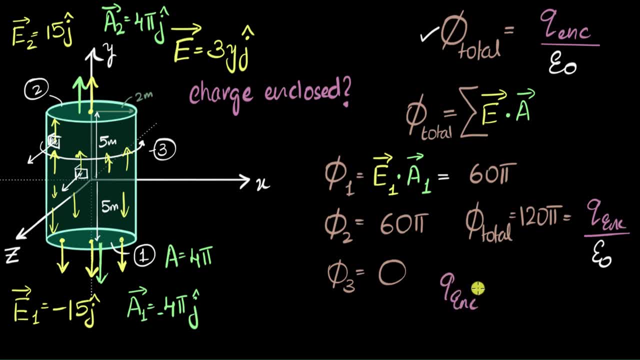 Charge enclosed equals: equals 120 pi times epsilon naught And we know the value of epsilon naught. we can plug that in and we get some answers and I'm pretty sure you can do that. But that's it, that's. I'm gonna stop over here. 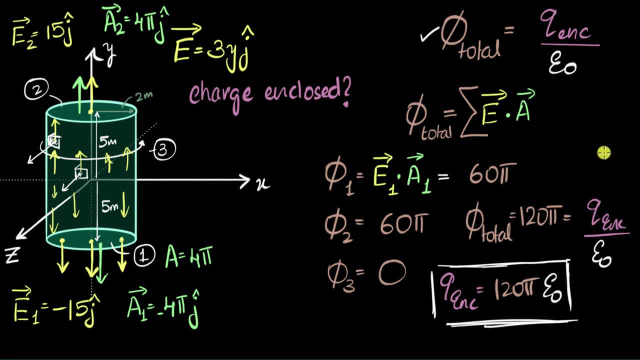 and we know how much charge is enclosed over here. And before I end I wanna give you a slightly different problem. My question to you is: what if we had everything exactly the same, except that the electric field was three times Modulus of y, times j cap? 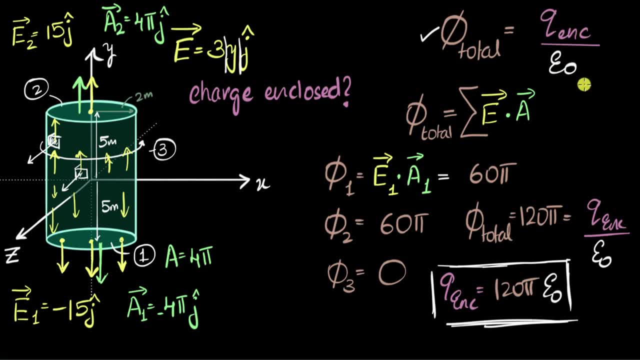 How would things change? What would be the new enclosed charge? Can you try and find this? It's not gonna take much time because most of the calculation is gonna stay the same. Okay, let's see if you did this. If you look at the top surface, everything would be the same. 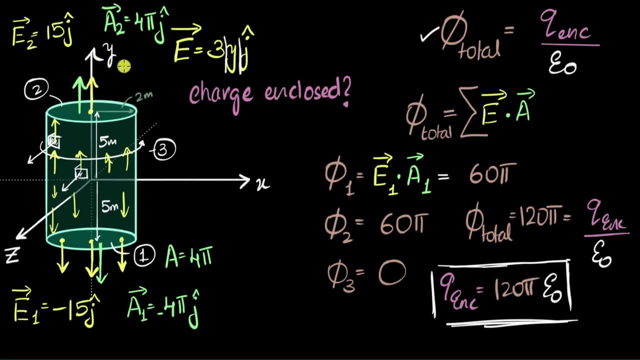 E2 would be just 15j. A2 vector would still be the same. you get the same answer. But this is where things will change. If I were to calculate E1, it's gonna be three times minus five, but the modulus of minus five. 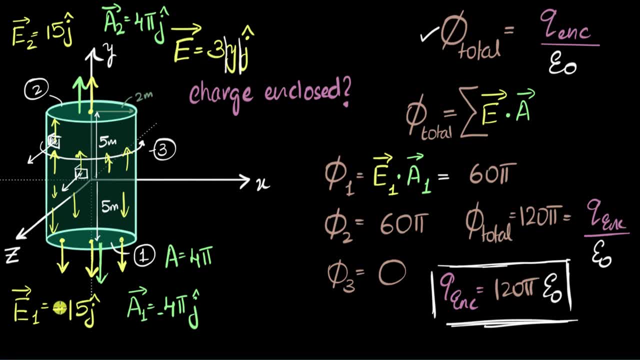 is plus five, so it's gonna be plus 15 over here in the second case. Which means now, in the second case, electric field is going to be pointing upwards, But your area vector is gonna be pointing downwards, because area vector should always be outwards. 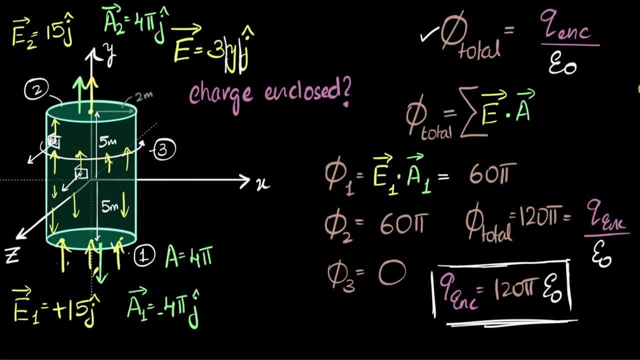 And therefore now when I calculate phi one, that's gonna be a negative 60. And see what you get. when you add up, you get zero. I mean curved surface will still remain zero, but the total flux will become zero. 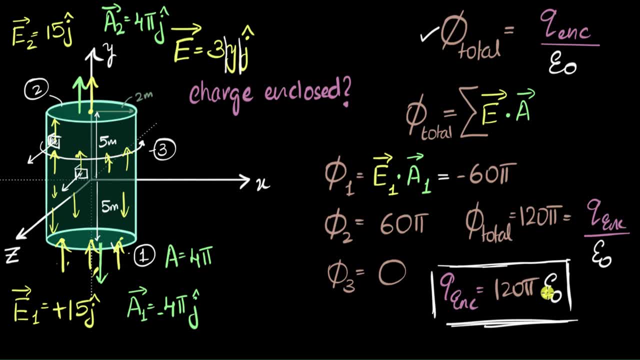 and the charge enclosed will now become zero.